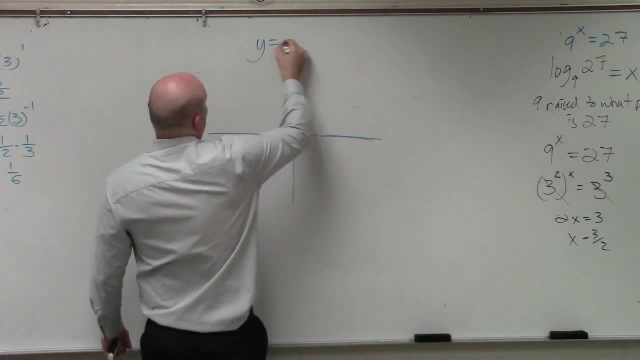 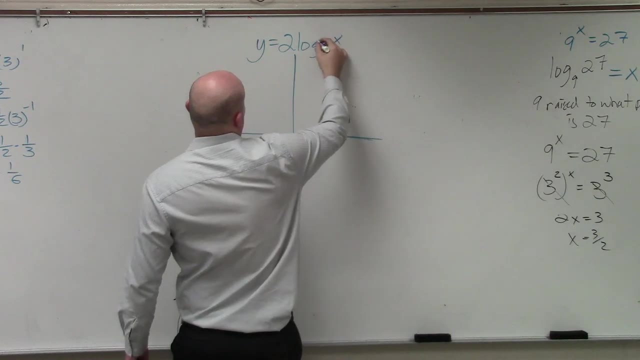 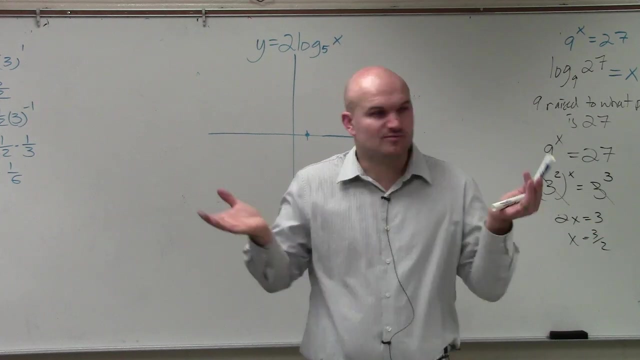 So they're asking us to graph: y equals 2 log. what was the base? There's base 5 of x, And then they really want you- oh they're saying- to find the domain and range, right? So really actually knowing what the graph is is really not that important right? 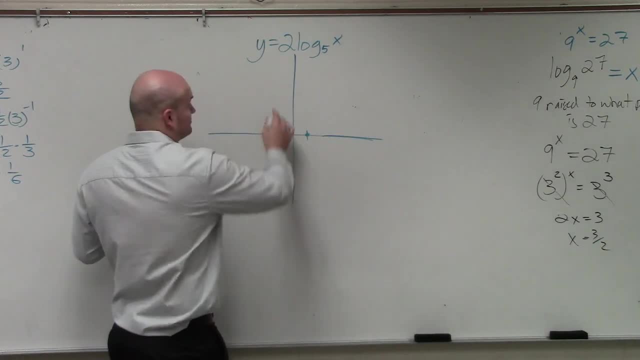 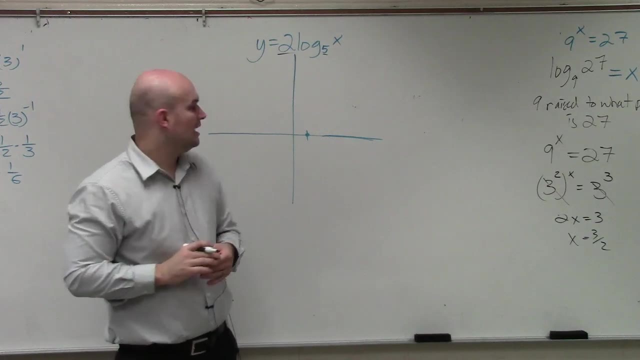 So, if you guys remember when we looked at this graph, when we looked at this graph, this actually did not, neither did these affect our transformations at all. They're not shifting your graph left or right, or up or down at all. 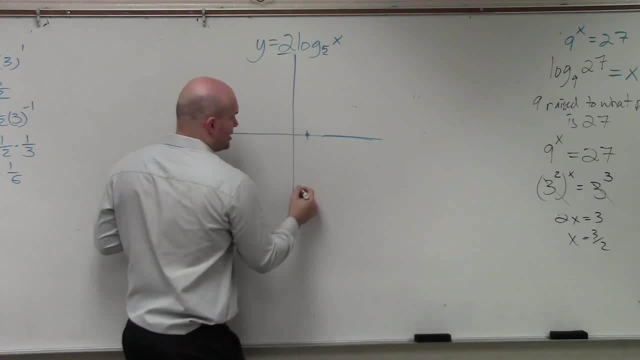 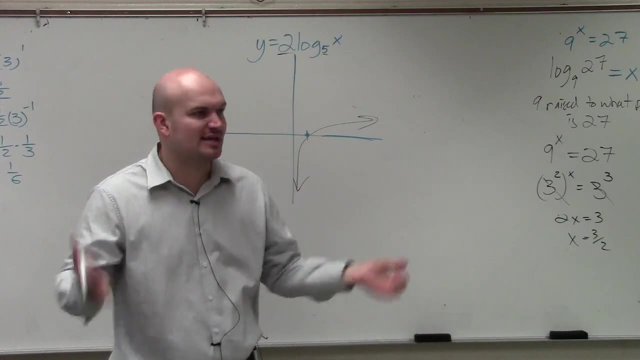 All these did, the graph still crosses at 1,, 0, and it just looks like this. You don't even need to have it perfectly correct. You don't even need to have the vertical stretch or compression or anything else, correct. We know that here this 2 is going to vertically stretch it. 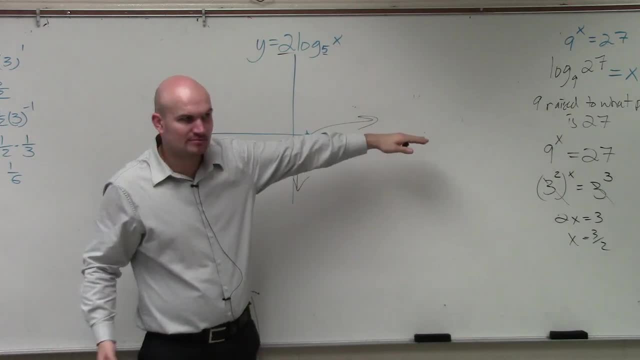 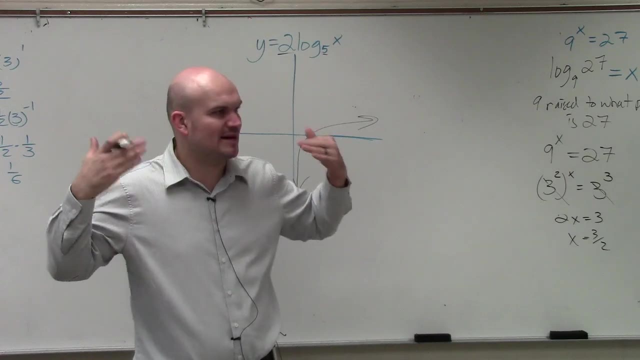 but this 5 actually makes it sharper turn okay, So it's actually kind of counterbalancing each other. But in reality they're not even asking for the graph. I'm just using the graph So I can visualize what the domain and range is. 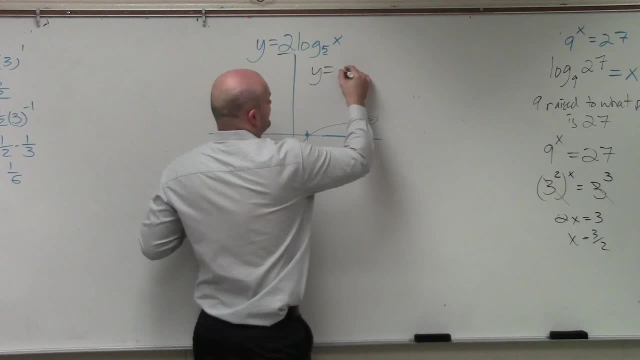 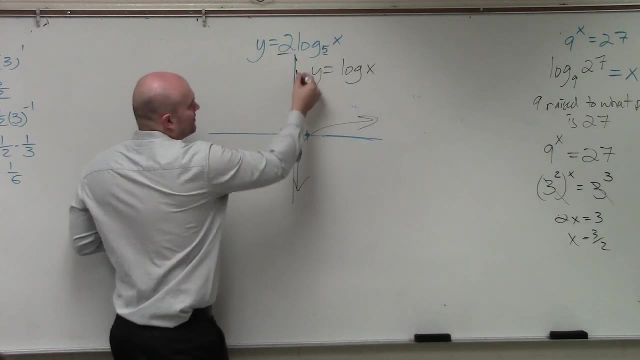 But do you guys notice? here's what the original parent graph would look like: Y equals, you know, log of X. There's no transformations, right? So remember, this graph has that asymptote, meaning this graph approaches 0, does not cross 0.. 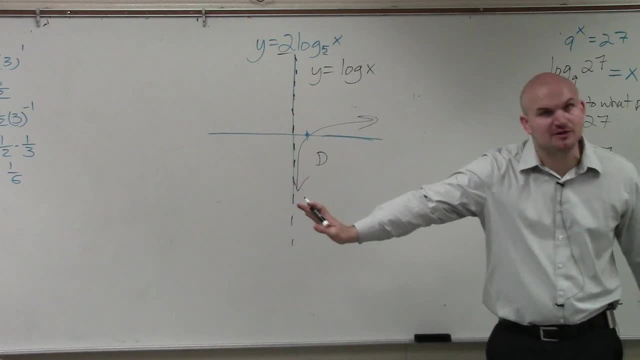 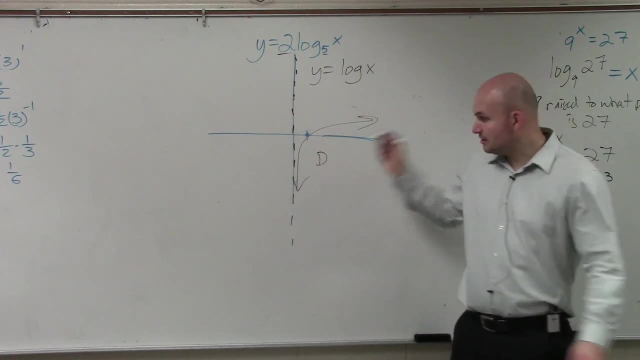 So the domain is basically asking us: how far left does this graph go to? how far to the right? So how far left does this graph go? How far to the left, To the right? Well Yeah, but it keeps on going down. 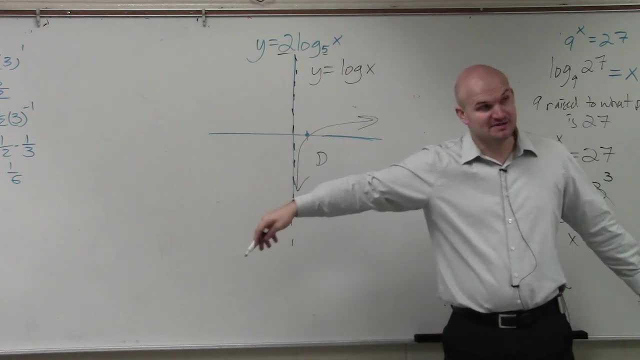 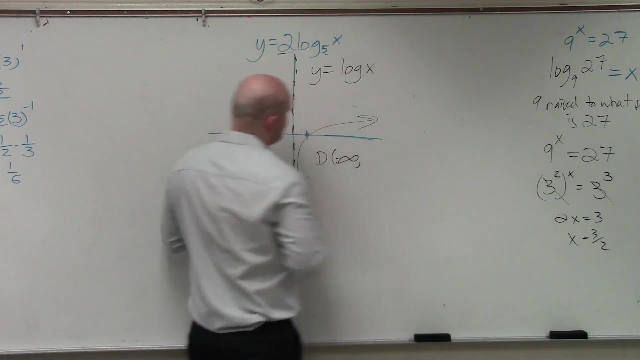 How far to the left is it going to go? 0.. Is it going to ever go to the other side of 0? No. Does it actually get on 0? No, Negative infinity. And then, how far to the right does it go? 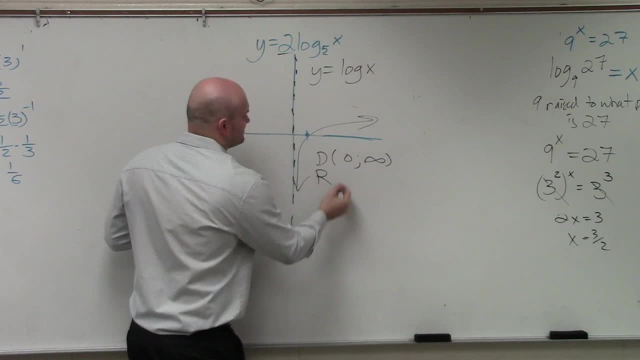 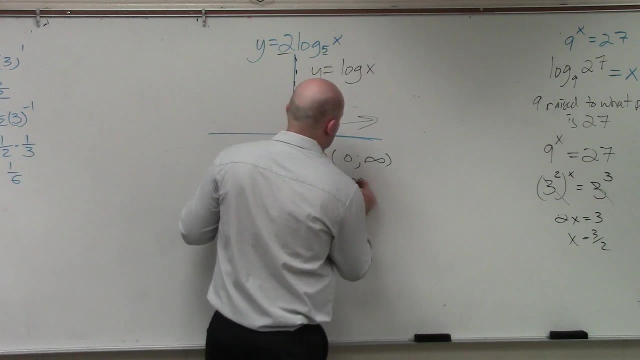 I'm sorry. 0, right. And then your range. Your range is negative infinity. A positive infinity, OK. Now the only thing I want you guys to understand for the other two equations. I said that the other two equations are not going to be positive infinity. They're going to go to, And so they are going to go to positive infinity. So they're not going to go to positive infinity, And so they're going to be positive infinity. You're going to ask what's the probability? When I was talking about that last time, there is a weird set of numbers. It's going to be like: oh, oh, it's because a lot of people are going to move a lot closer to each other, and so maybe they're going to move a lot closer to each other.